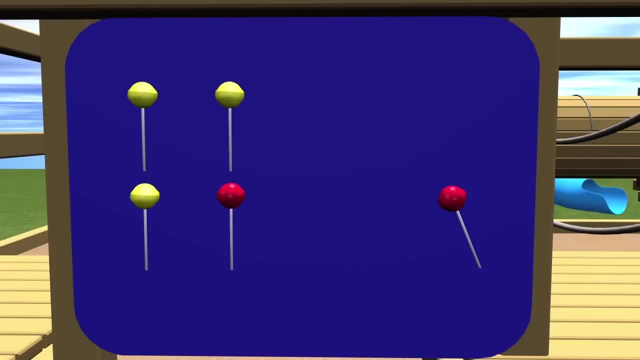 going to take these two and put them into a pair, And then I'm going to put this one into a Wait, I can't put this piece of candy into a pair. There's not another piece of candy to put it with. Since I cannot put this into another pair, I realize that this is an odd number. 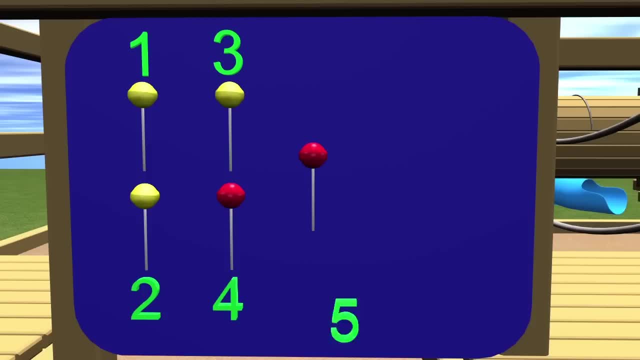 So 1,, 2,, 3,, 4,, 5 is an odd number. I have 2 here, 2 here and 1 all by itself, 5 is an odd number. Let's take a look at this whiteboard and see how many even or odd magnets we have. 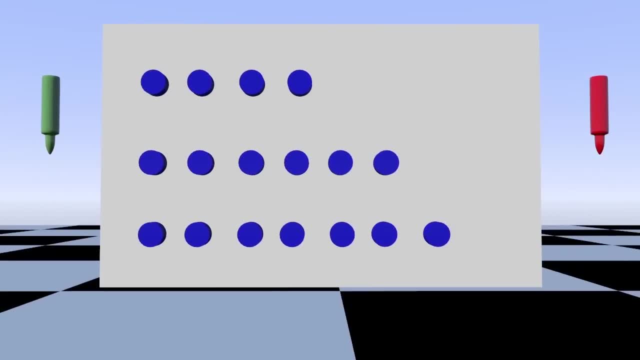 Wait, I can't move these magnets, It's too strong. It looks like we're going to have to think of another way to figure out the even and odd numbers. I have an idea: I can put them into pairs by adding a circle around 2s. when we find 2s, 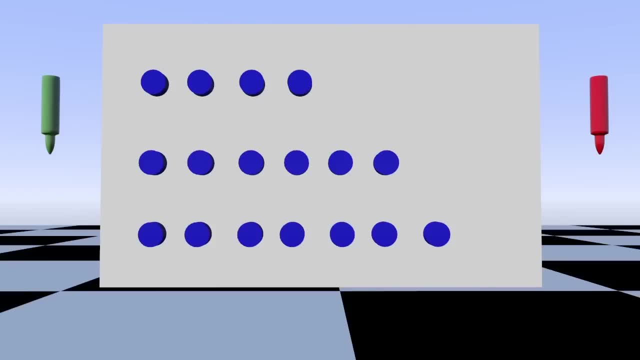 Let's do that together. Let's look at this top row right here and count how many magnets we have. Here's 1,, 2,, 3, 4.. Let's go ahead and put them into pairs. This is a pair and this is a pair. 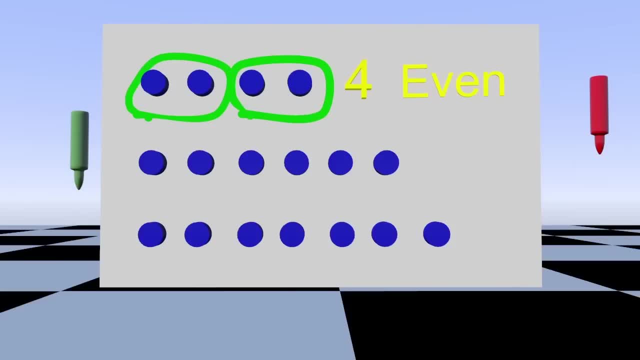 So 4 is an even number because it can be put into equal pairs. Let's look at the next row. Here's 1, 2, 3, 4.. 5, 6.. Some of you are probably already catching on and you can tell right away. 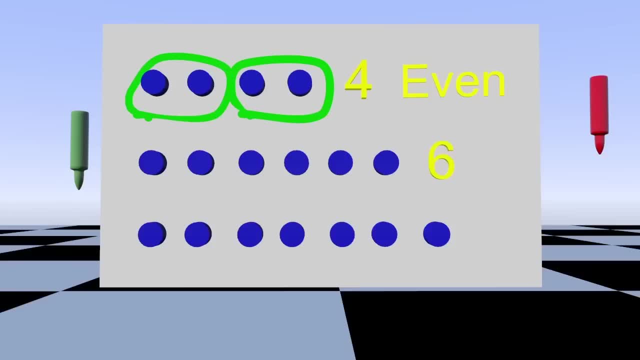 Is this an even or odd number? Well, let's see. Let's put these into pairs and figure out if this is going to be even or odd. Let's circle these two and these two and these two. Look, If you said even, then you are right, because they can all be put into pairs. 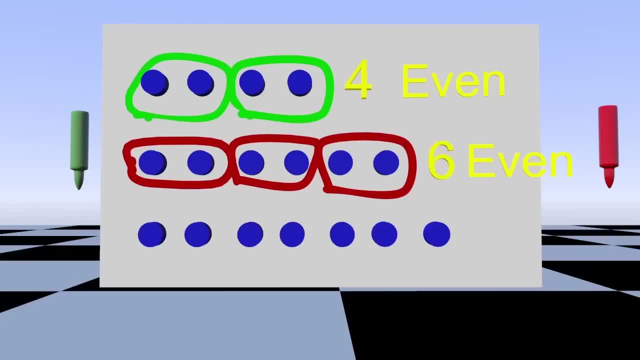 Great job. There are 6 magnets here that can be put into pairs, and that makes 6 an even number. Now let's look at this last row. Here's 1, 2, 3, 4, 5, 6, 7.. 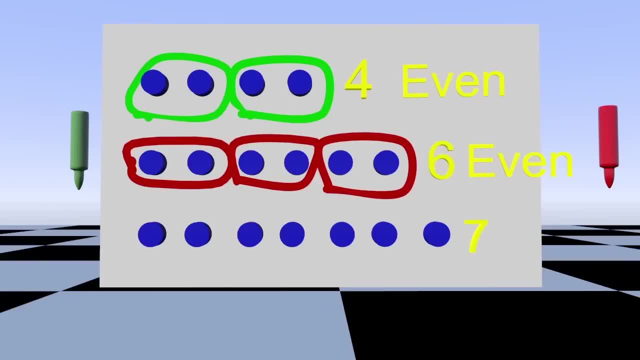 Let's go ahead and put these into pairs to see if we have an even or odd number. Let's put these two together, and these two together, and these two together. and Uh-oh, We can't put this into a pair because there's not another magnet to pair it with.